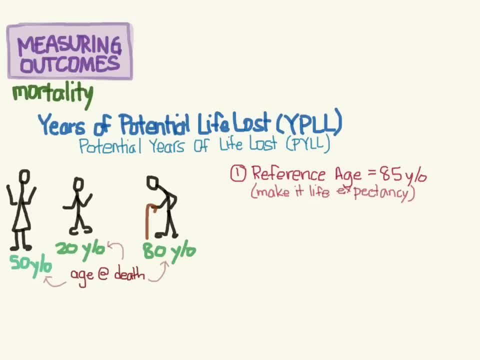 So once you've picked your reference age- and it makes sense to pick the life expectancy for this population- then you're going to subtract the age of death from the reference age. So we have one person dying at 80.. We have one person dying at 20 and another one dying at 50, and so that's going to be 5, and then 65 and 35.. 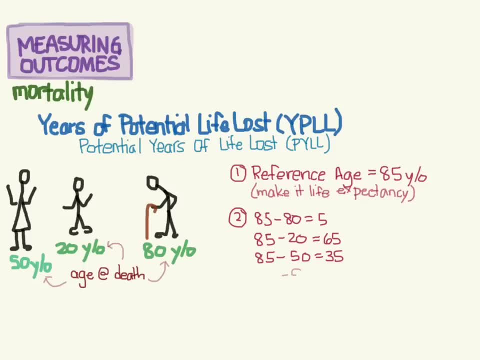 Now let's say we had someone who died at age 92. Okay, so we had another person here, 85 minus 92. And then that would be negative 75. But for the purposes of these calculations we don't have negative numbers, to just count that as zero. 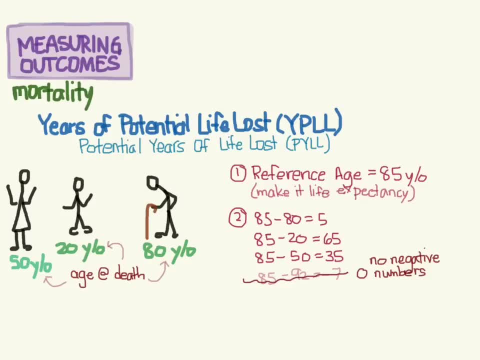 Because really, what are we doing? We want to see how much above the reference age this person lived- and this one didn't live, lived past the reference age, so they didn't die prematurely- And so we want to calculate all these differences here, and then you simply just add them up. 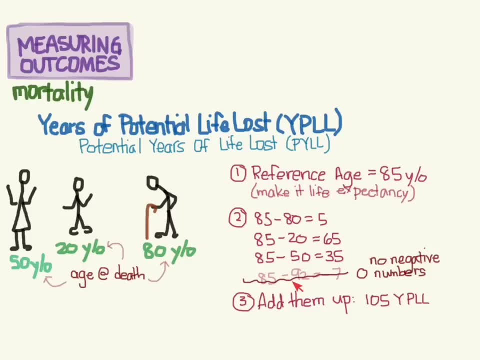 So for this particular group of- well, we could say- four people, we have 105 years of potential life lost. So you can see that if a younger person dies prematurely, their loss contributes more to this value. So this is really good at focusing on things that kill young people. 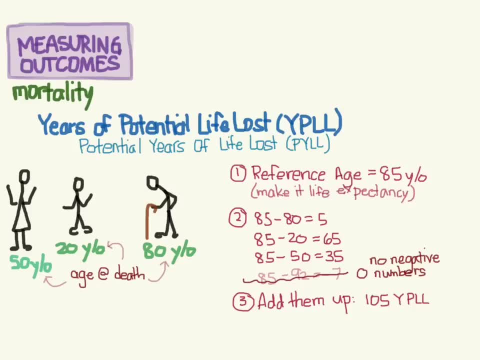 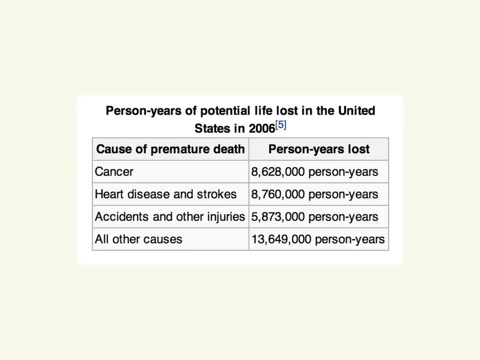 So if you want to emphasize the things that kill younger people, you can use years of potential life lost And you can look at all-cause mortality, meaning all deaths, or you could even look at deaths due to specific causes. And so here we are looking at the years of potential life lost and we're looking at four different etiologies here. 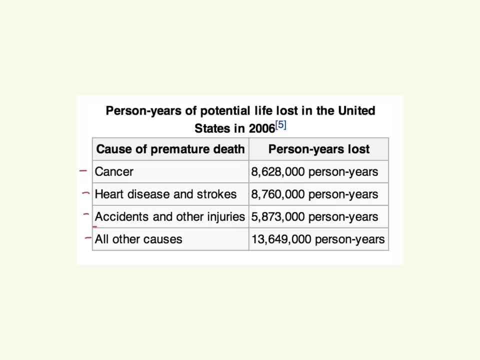 Well, really three, and then one bucket that looks at a bunch, that looks at all the other causes, And so you can see that things that are going to kill younger people you tend to be more likely to die prematurely. You tend to be have more weight. 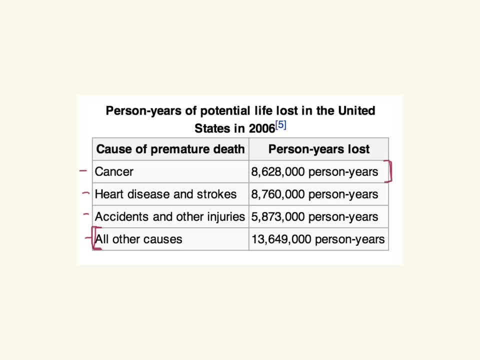 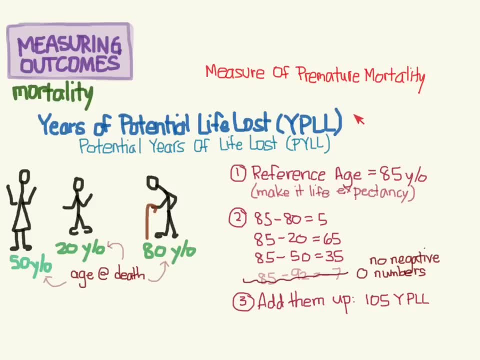 And so cancer is going to kill more people than heart disease, And so then, cancer is a bigger number. So that's years of potential life lost. Y-P-L-L as a measure of premature mortality- See you in the next video.